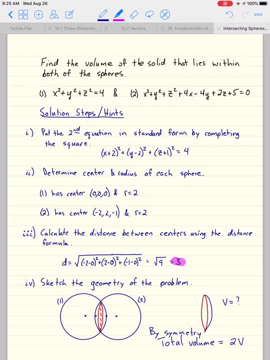 Okay, So the distance of 3 between the two centers, it's a nice whole number distance. It kind of begs us to draw, or at least sketch, what the geometry of this problem looks like. Now, one thing I would encourage is: don't try to sketch this sphere exactly where it is in a 3-dimensional coordinate system. 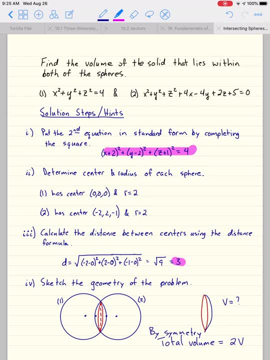 That's just going to be difficult. Right, We can use the distance between these two spheres. The fact that they have the same radius tells us that they have the same shapes, So we can just really get a cross-sectional view of these two spheres' intersections. 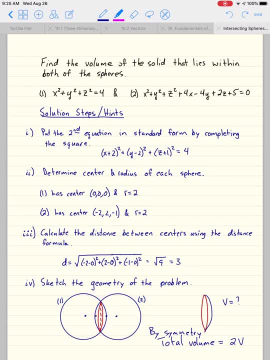 And that's what I've got right here. This is the 2-dimensional view of the intersection of these two spheres, These two 3-dimensional spheres. So just to zoom in a little bit, Um, and the way I've drawn it. 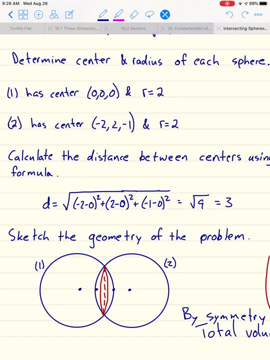 Um, and the way I've drawn it is not to try to figure out where they are in 3 dimensions and really work on a plane that passes through these two. But of course, yes, there is a plane represented right here that passes through these two spheres. 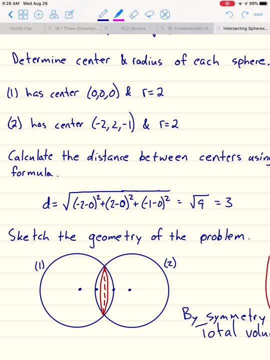 We don't have the tools to establish the equation of that plane yet, So there must be a simpler way through this. In fact there is. So the way I've drawn these two circles or two spheres in profile, just looking at them as a slice, 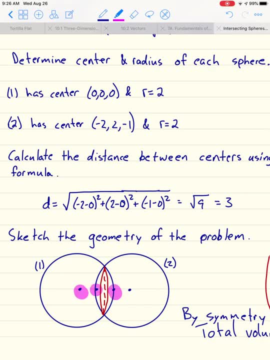 is to mark off 1, 2, 3.. These four points are unit distances apart. So stepping from this center of circle 1, step 1, 2 units is the outside edge of that sphere or circle in profile. 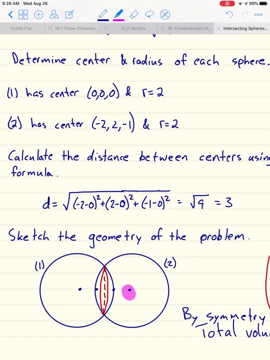 Going the other way, we've got 1,, 2 units to represent the radius of the other sphere in profile. Now, in between, is this line right here? Okay, so halfway between these? well, if we, you know, needed to really calculate that. 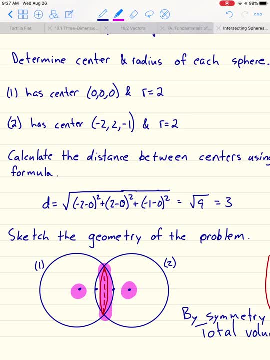 we'd realize that these two centers are 3 units apart. Halfway between them is a distance of 1 and a half, So what we know now is that this line here is actually 1 and a half units away from each center, And what we're looking for then. 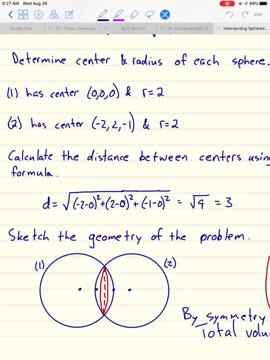 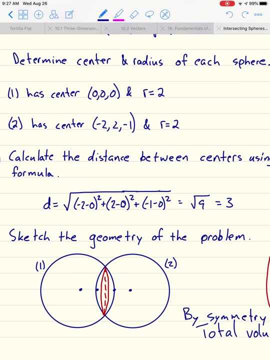 is the volume of the end cap of a sphere when this flat portion here, this flat portion here, is at the point 1 and a half units. its center point is 1 and a half units away from the center of the sphere. 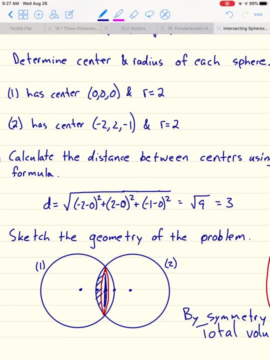 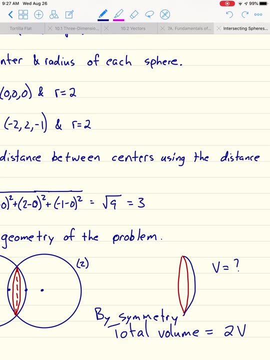 and we're looking at the volume of the rest of the end cap this way, Okay. so to clean that up again, we'll see the picture drawn off to the side. We're just looking at the volume of a piece like this, Okay, and so that's only half of them. 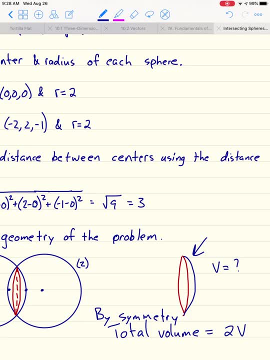 that's one end cap, but since they're symmetric, the two spheres both have radius 2, then we'll just double the volume that we find here to get the total volume. So how do we find the volume of the end cap of a sphere? 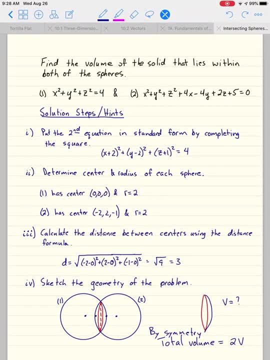 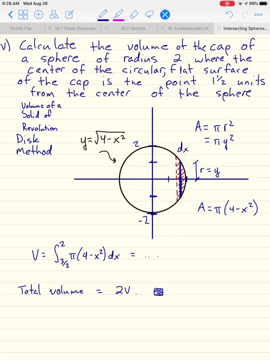 Well, we'll have to remember calc 2.. We'll go back to calc 2 techniques: volume of a solid of revolution, that's step 5, and we'll calculate the volume of that end cap. So what I've done now is just taken one circle. 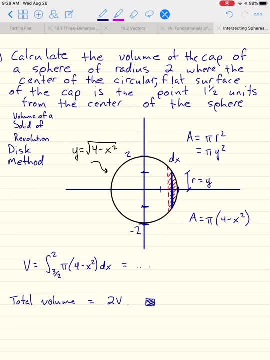 that we're going to rotate about. I don't know, it doesn't really matter whatever axis we rotate this circle about, but maybe we'll say this axis, the x axis. Okay, that'll form a sphere If we look at just this line right here. 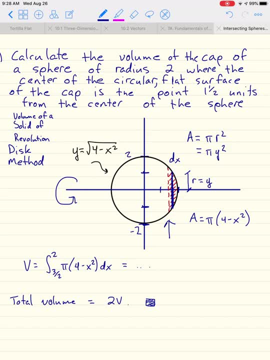 that'll form the end cap that we're interested in and from what follows. this way, we're just going to use the disc method for the volume of a solid of revolution and it's just essentially calc 2 techniques. Remember that the radius at any given point 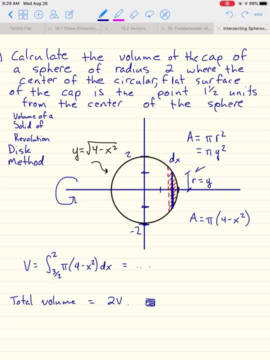 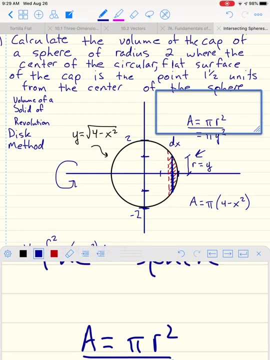 is given by this little segment. here, If we're looking at cross-sectional areas of these discs, the area's going to be a equals pi r squared. Remember that the volume formula tells us that we're going to need to use v equals a to b. 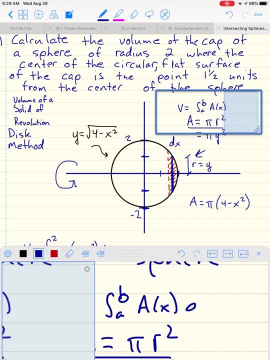 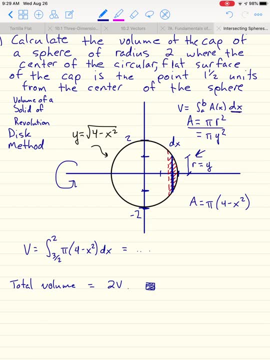 some limits of integration. a of x, dx, and that's how we sum up all the areas times, their infinitesimal widths, dx, to get the volume of this solid of revolution. for this end. cap Now some things we know about this.